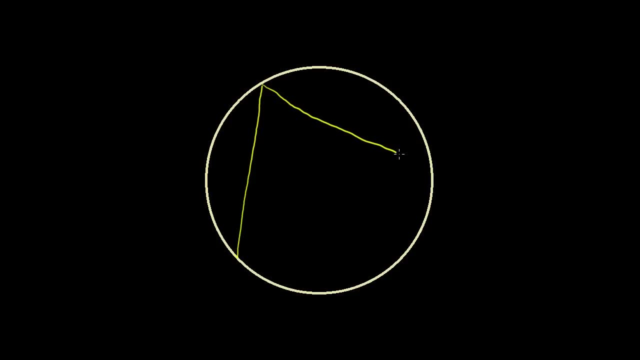 So I'm going to try my best to draw an equilateral triangle. I think that's about as good as I'm going to be able to do. And when I say equilateral, it means all of these sides are the same length. So if this is side length a, then this is side length a. 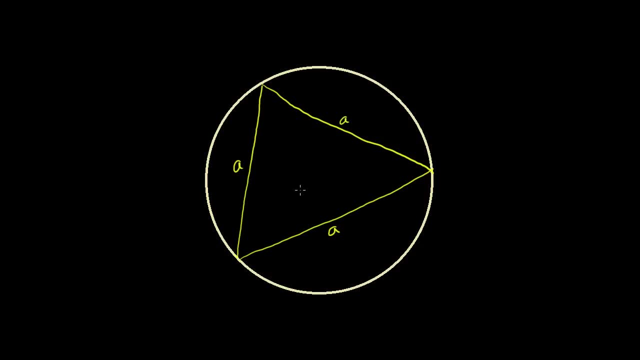 And that is also a side of length a. And let's say we know that the radius of this circle is 2.. I'm just picking a number just to do this problem. So let's say the radius of this circle is 2.. 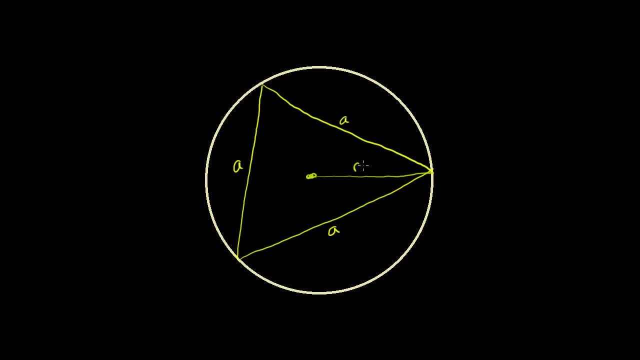 So, from the center to the circumference, at any point, this distance, the radius, is equal to 2.. Now what I'm going to ask you is using some of what we've learned so far, what we've used in the results of the last few videos. 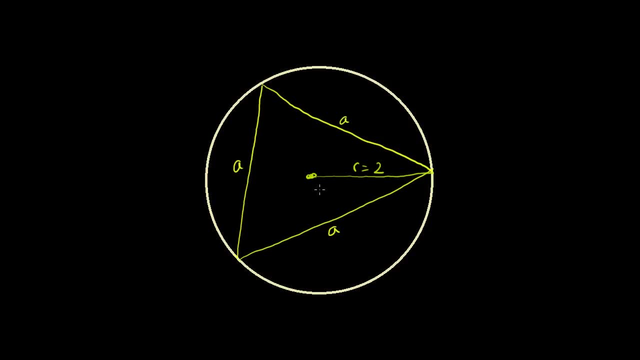 and a little bit of basic trigonometry, And if the word trigonometry scares you, you'll just need to know maybe the first two or three videos in the trigonometry playlist to be able to understand what I do here. What I want to do is figure out the area of the region. 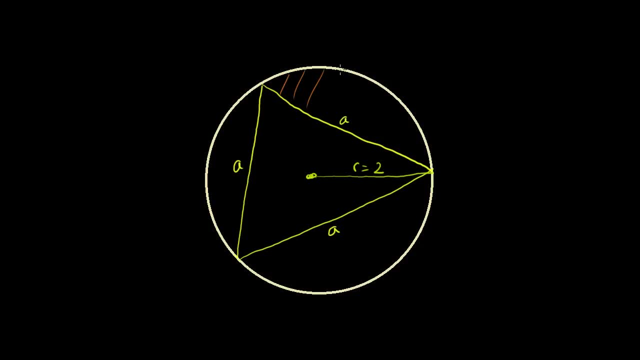 inside the circle and outside of the triangle. So I want to figure out the area of that little space, that space and this space. So the obvious way to do this is to say: well, I can figure out the area of the circle pretty easily. 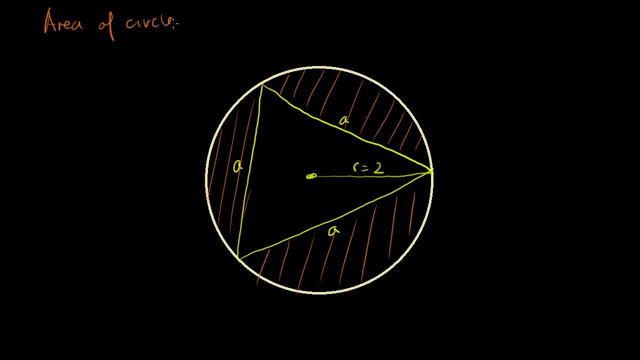 Area of the circle. That's going to be equal to pi r squared, or pi times 2 squared, which is equal to 4 pi, And I could subtract from 4 pi the area of the triangle. So we need to figure out the area of the triangle. 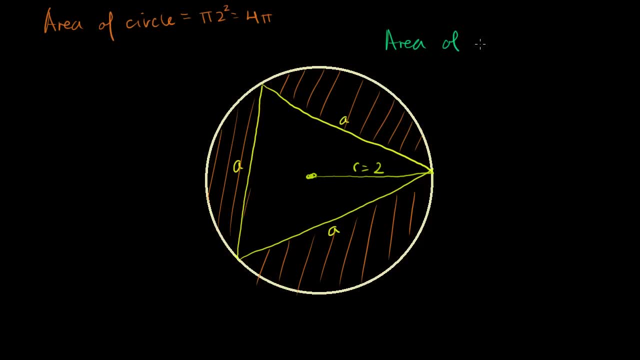 What is the area of the triangle? The area of the triangle? Well, from several videos ago I showed you Heron's formula where, if you know the lengths of the sides of a triangle, you can figure out the area, But we don't know the lengths of the sides just yet. 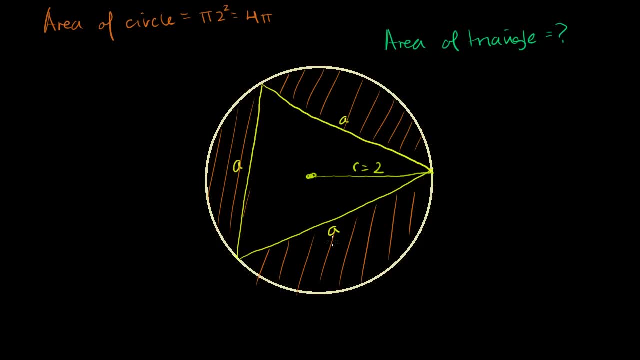 Once we do, maybe we can figure out the area. Let me apply Heron's formula not knowing it. So let me just say that the lengths of this equilateral triangle, the lengths of the sides, are a Applying Heron's formula. so let me do Heron's right here. 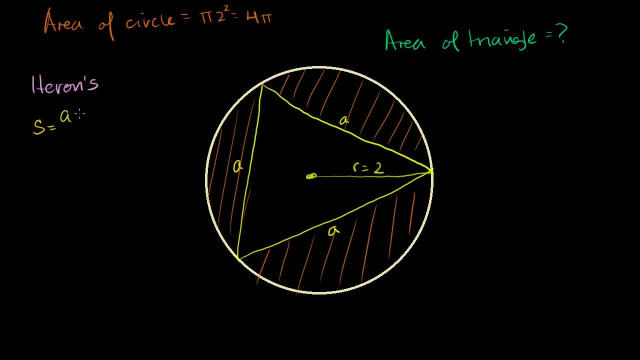 we first define our variable s as being equal to a plus a, plus a over 2,, or that's the same thing as 3a over 2.. And then the area of this triangle in terms of a. so the area is going to be equal to the square root of s. 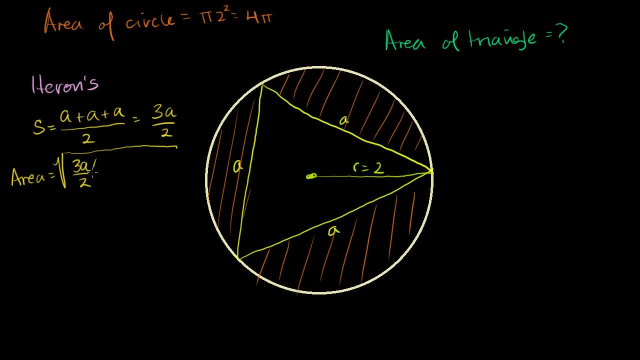 which is 3a over 2, times s minus a. So that's 3a, 3a over 2 minus a, Or I could just write 2a over 2.. a is the same thing as 2a over 2.. 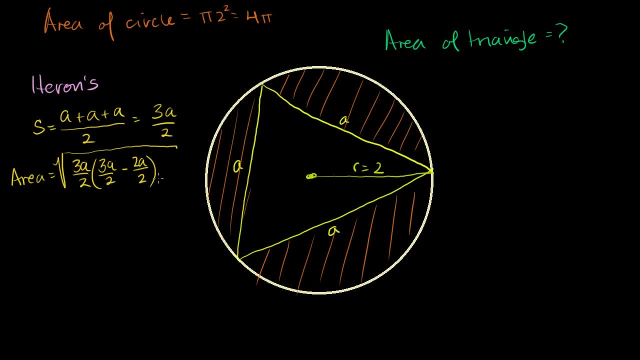 You could cancel those out and get a, And then I'm going to do that three times. So instead of just multiplying that out three times for each of the sides, by Heron's formula, I could just say to the third power: So what's this going to be equal to? 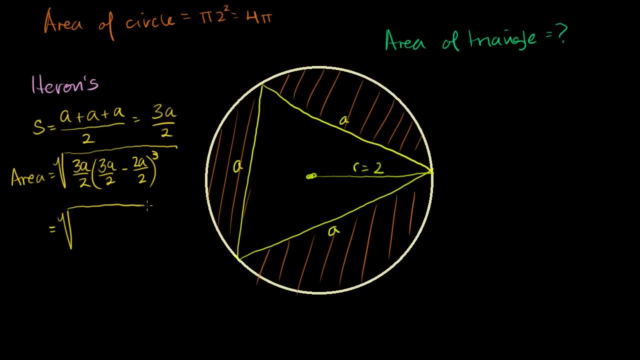 This is going to be equal to the square root of 3a: 3a over 2.. And then this right here is going to be equal to: 3a minus 2a is a. So a over 2 to the third power. 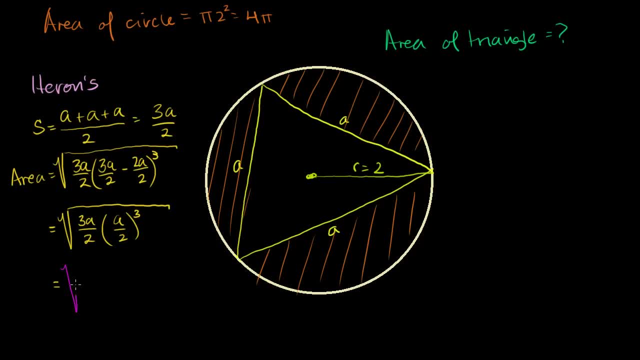 And so this is going to be equal to. I'll arbitrarily switch colors. We have 3a times a to the third, which is 3a to the fourth, over 2 times 2 to the third. Well, that's 2 to the fourth. 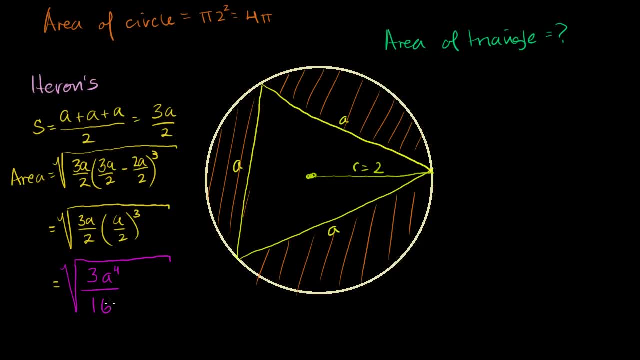 That's the fourth, power, or 16.. 2 times 2 to the third is 2 to the fourth, That's 16.. And then, if we take the square root of the numerator and the denominator, this is going to be equal to the square root of a to the fourth. 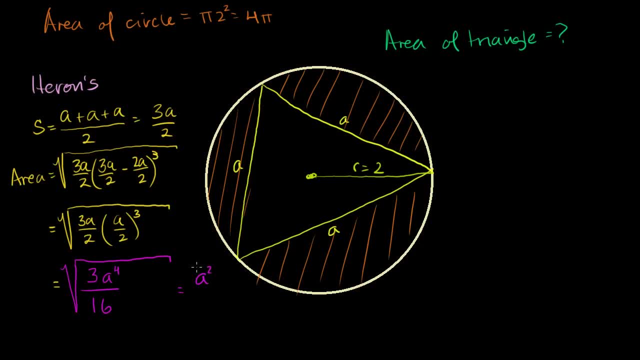 is a squared times. well, I'll just write the square root of 3 over the square root of the denominator, which is just 4.. So if we know a using Heron's formula, we know What the area of this equilateral triangle is. 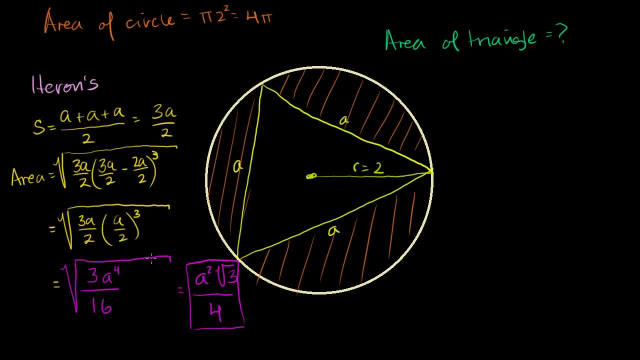 So how can we figure out a? So what else do we know about equilateral triangles? Well, we know that all of these angles are equal And since they must add up to 180 degrees, they all must be 60 degrees. That's 60 degrees. 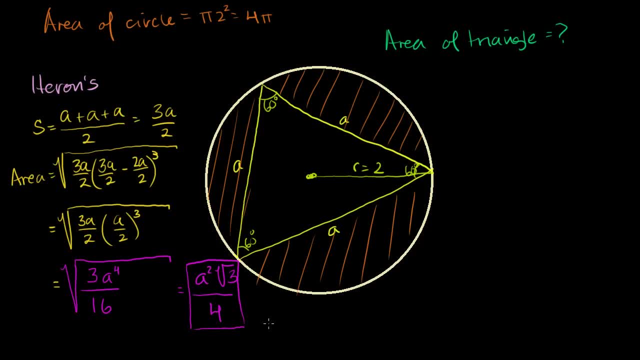 That's 60 degrees. And that is 60 degrees. Now let's see if we can use the last video where I talked about the inscribed, The relationship between an inscribed angle and a central angle. So this is an inscribed angle, right here. 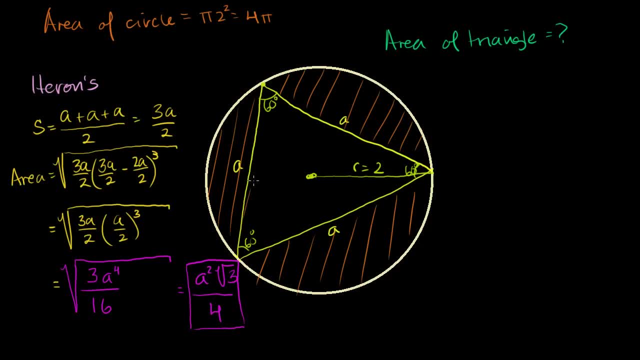 It's a vertex, It's sitting on the circumference And so it is subtending this arc right here. It is subtending that arc right there And the central angle that is subtending that same arc is this one right here, The central angle subtending that same arc. 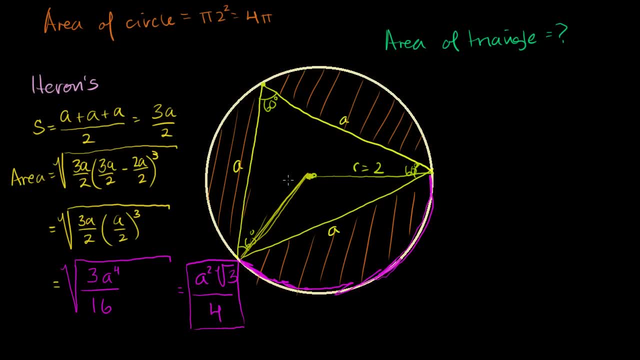 is that one right there? So, based on what we saw in the last video, the central angle that subtends the same arc is going to be double of the inscribed angle. So this angle right here is going to be 120 degrees. Let me just put an arrow there. 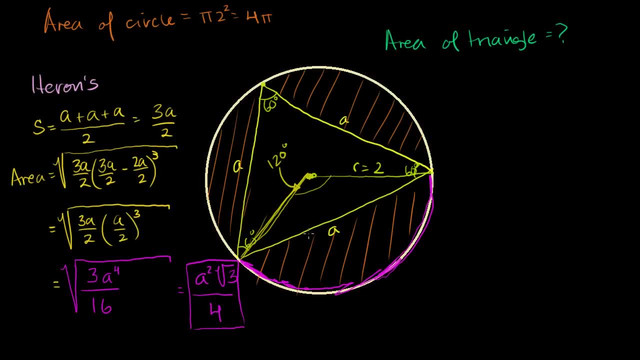 120 degrees, It's double of that one. Now, if I were to exactly bisect this angle right here, so I go halfway through the angle and I would just go straight down, straight down, like that, What are these two angles going to be? 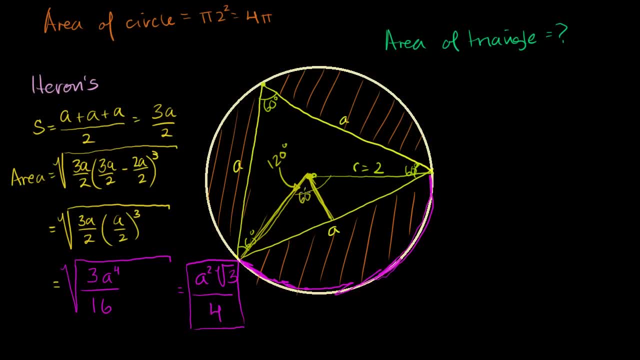 Well, they're going to be 60 degrees. I'm bisecting that angle. That is 60 degrees and that is 60 degrees right there, And we know that I'm splitting this side in two. This is an isosceles triangle. 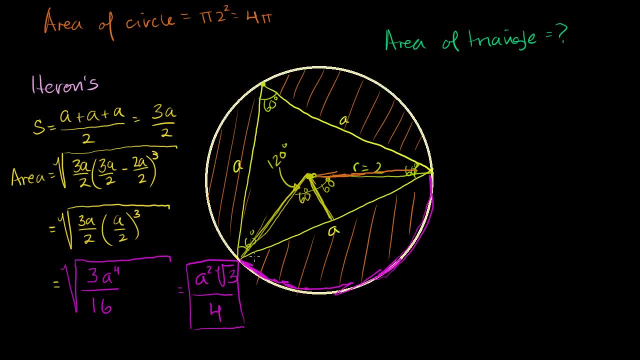 This is a radius right here. Radius r is equal to 2.. This is a radius right here of r is equal to 2.. So this whole triangle is symmetric. If I go straight down the middle, this length right here, This length right here, is going to be that side divided by 2.. 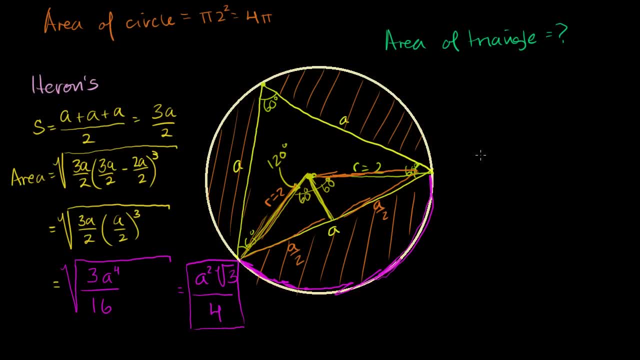 That side right, there is going to be that side divided by 2.. Let me draw that over here. If I just take an isosceles triangle, any isosceles triangle where this side is equivalent to that side, Those are our radiuses in this example. 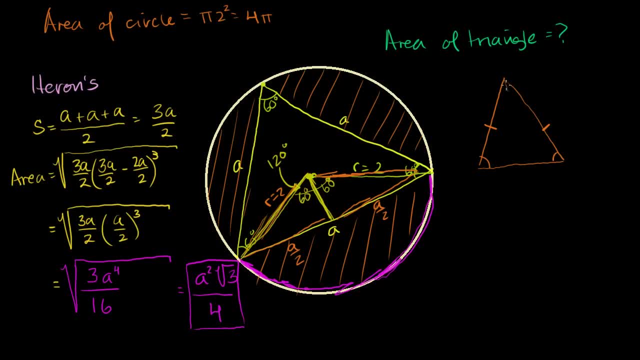 And this angle is going to be equal to that angle. If I were to just go straight down this angle right here, I would split that opposite side in two, So these two lengths are going to be equal In this case. if the whole thing is a, 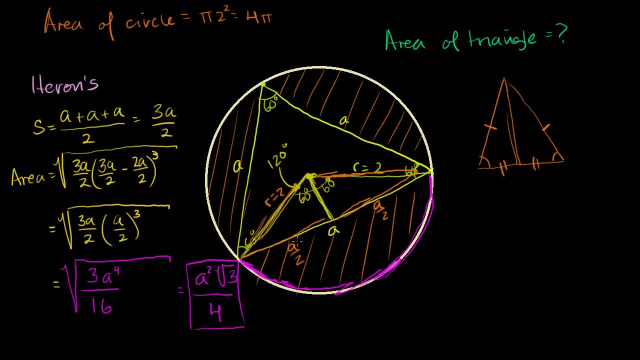 each of these are going to be a over 2.. Now let's see if we can use this and a little bit of trigonometry to find a relationship between a and r, Because if we're able to solve for a using r, 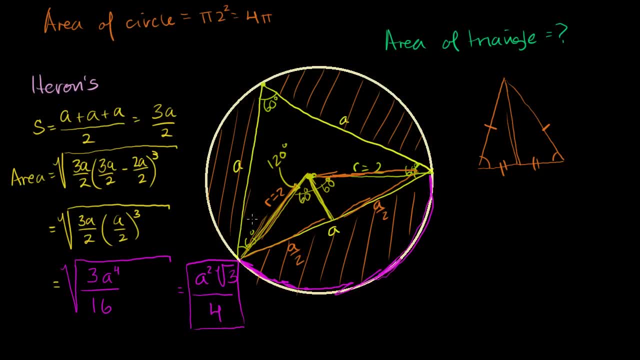 then we can then put that value of a in here And we'll get the area of our triangle And then we could subtract that from the area of the circle And we will have been done. We will have solved the problem. So let's see if we can do that. 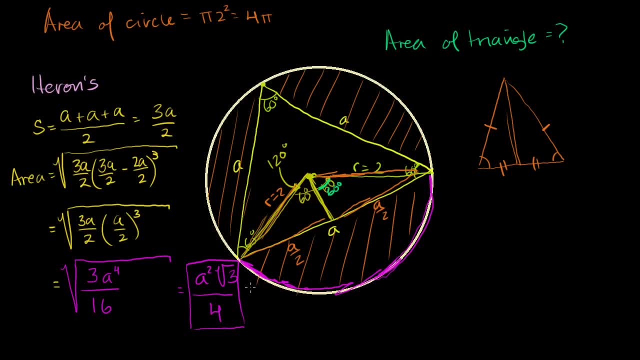 So we have an angle here of 60 degrees. 60 degrees, half of this whole central angle right there. If this angle is 60 degrees, we have a over 2. That's opposite to this angle. So we have an opposite. 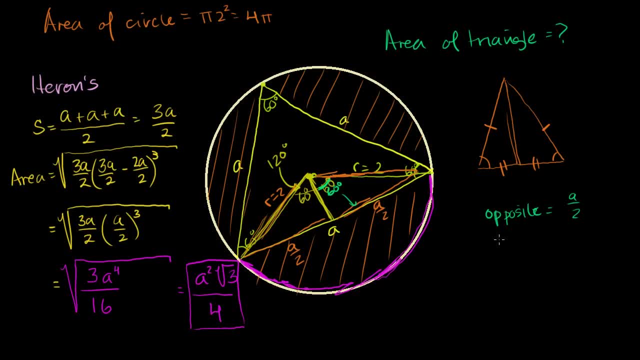 Opposite is equal to a over 2.. And we also have the hypotenuse. This is a right triangle. right here You're just going straight down and you're bisecting that opposite side. This is a right triangle, So we can do a little trigonometry. 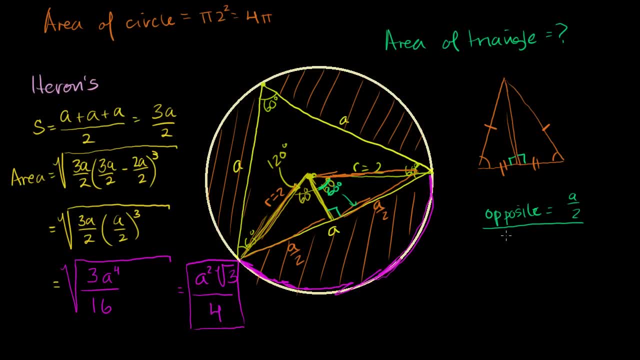 Our opposite is a over 2.. The hypotenuse: The hypotenuse is equal to r. This is the hypotenuse right here of our right triangle. So that's equal to 2.. So what trig ratio is the ratio of an angle's opposite side? 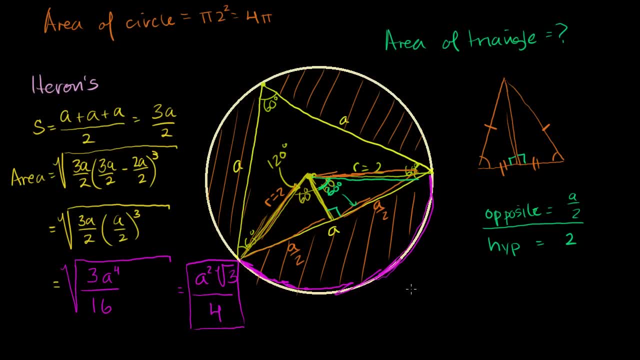 to hypotenuse. So some of y'all might get tired of me doing this all the time, But SOH CAH TOA. So sine of an angle is equal to the opposite. over the hypotenuse. Let me scroll down a little bit. 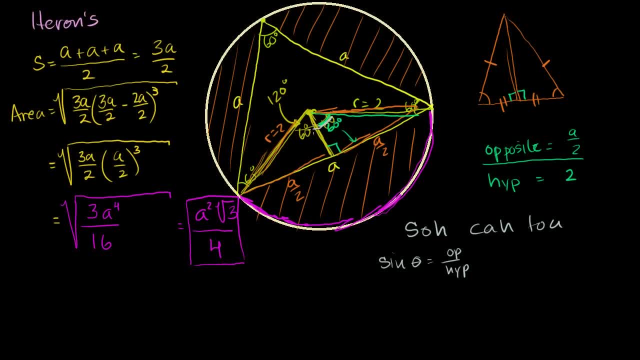 I'm running out of space. So the sine of this angle right here, the sine of 60 degrees, is going to be equal to the opposite side, is going to be equal to a over 2 over the hypotenuse, which is our radius over 2, which is equal to a over 2 divided by 2. 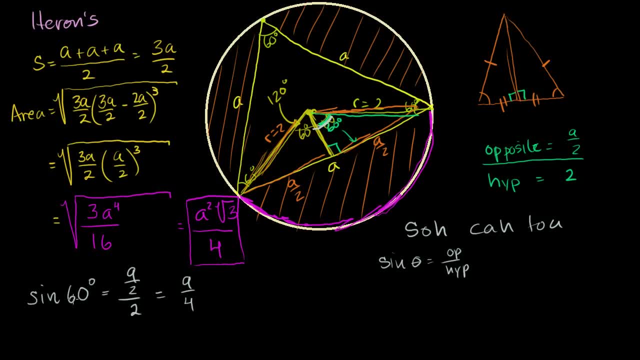 is a over 4.. And what is sine of 60 degrees? And if you don't, If the word sine looks completely foreign to you, watch the first several videos on the trigonometry playlist. It shouldn't be too daunting. Sine of 60 degrees, you might remember from your 30-60-90. 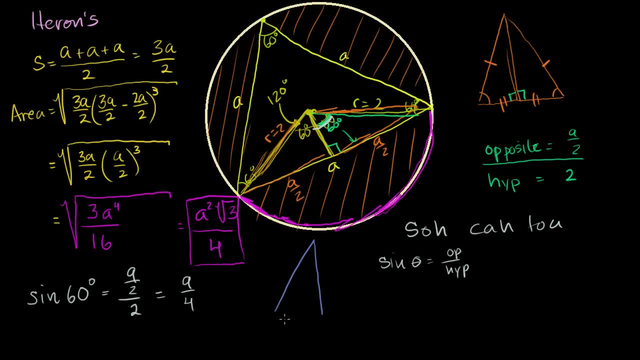 triangles. Let me draw one right there. So that is a 30-60-90 triangle. If this is 60 degrees, that is 30 degrees, That is 90. You might remember that this is of length 1.. This is going to be of length 1 half. 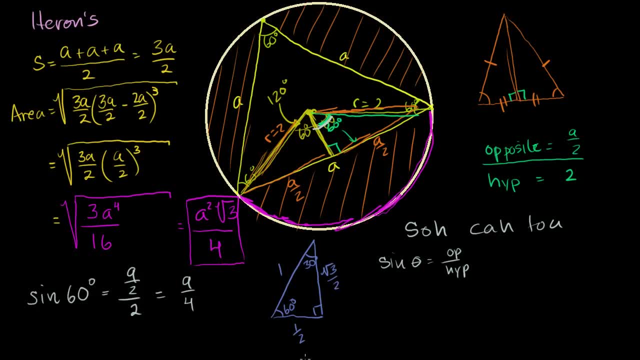 And this is going to be of length- square root of 3 over 2.. So the sine of 60 degrees is opposite over hypotenuse. Square root of 3 over 2 over 1.. Sine of 60 degrees if you don't have a calculator. 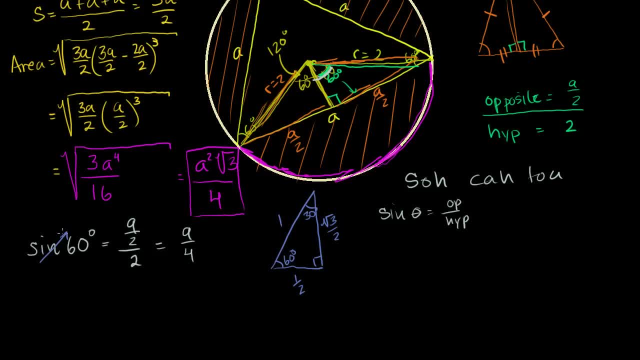 you could just use. this is square root of 3 over 2.. So this right here is square root of 3 over 2.. Now we can solve for a Square root of 3 over 2 is equal to a over 4.. 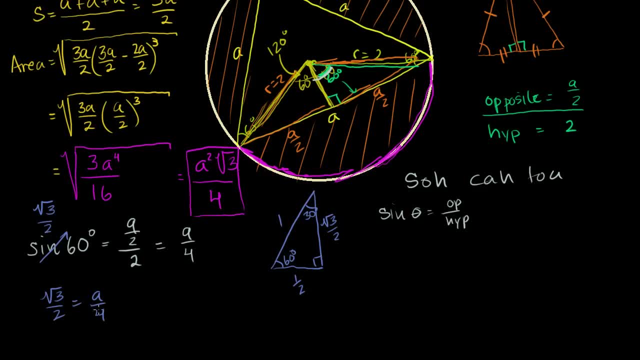 Let's multiply both sides by 4.. So you get this. 4 cancels out. You multiply 4 here. This becomes a 2. This becomes a 1. You get a is equal to 2 square roots of 3.. 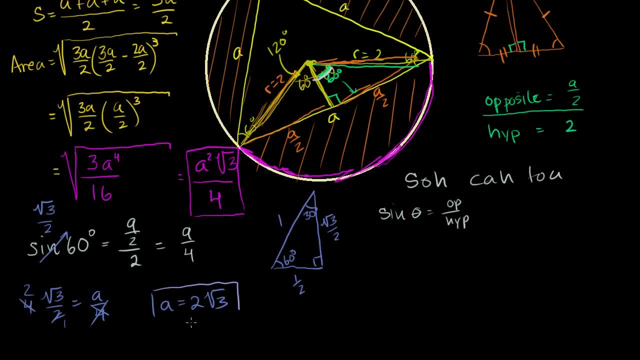 We're in the home stretch. We just figured out the length of each of these sides. We used Heron's formula to figure out the area of the triangle in terms of those lengths. So we just substitute this value of a into there to get. 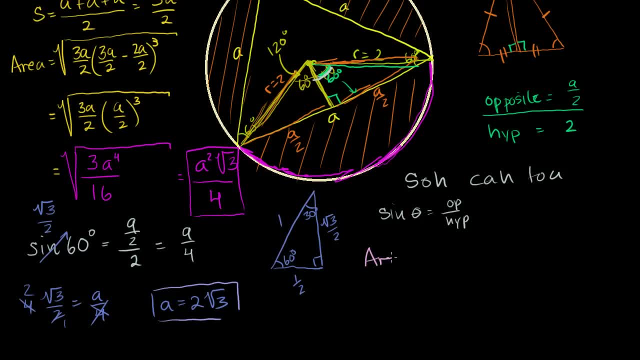 our actual area. So our triangle's area Is equal to a squared. What's a squared? That is 2 square roots of 3 squared times the square root of 3 over 4.. We just did a squared times the square root of 3 over 4.. 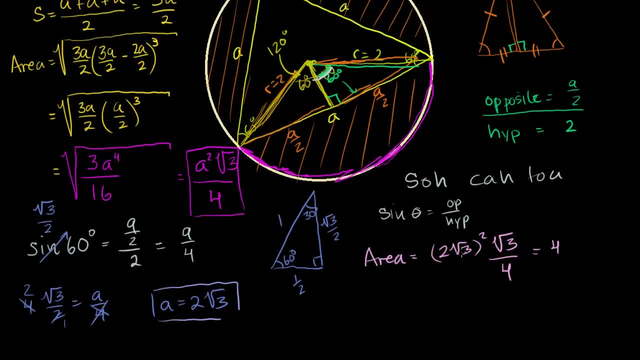 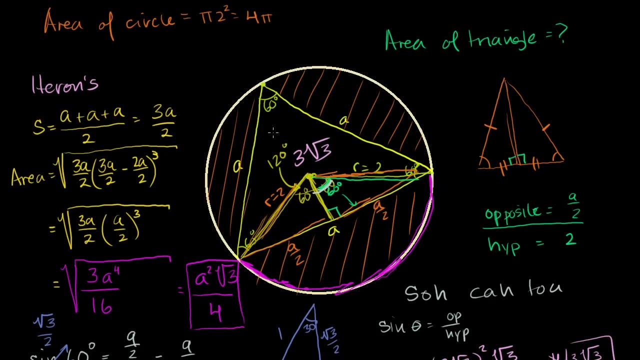 This is going to be equal to 4 times- 3 times the square root of 3 over 4.. These 4's cancel, So the area of our triangle We got is 3 times the square root of 3.. So the area here is 3 square roots of 3..